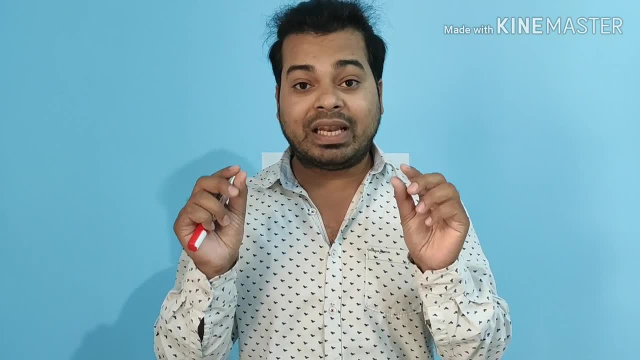 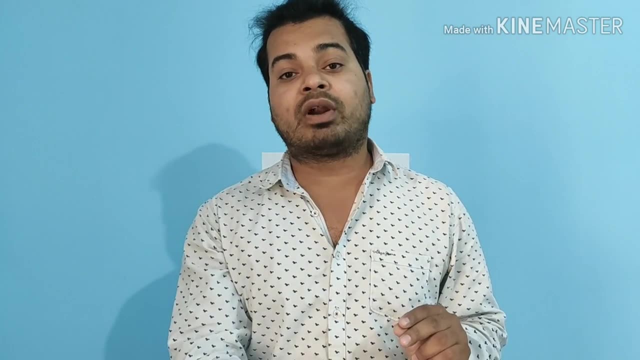 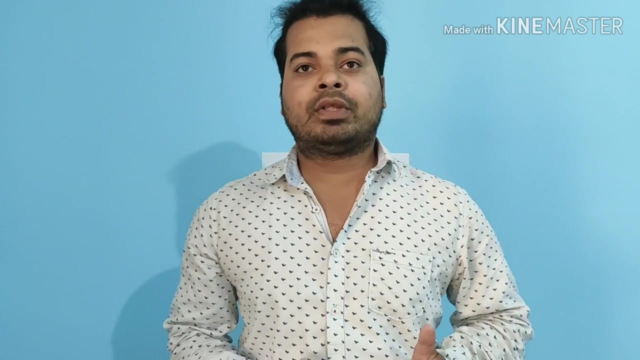 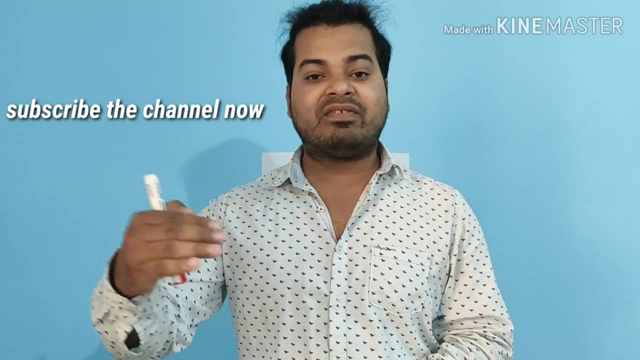 less about software development lifecycle. I'm going to mainly concentrate about what are the advantages and disadvantages of choosing a waterfall model as a software development lifecycle. So let's get started. So in the waterfall model as a software development lifecycle, there are many seven phases. The first is: let me teach you guys. 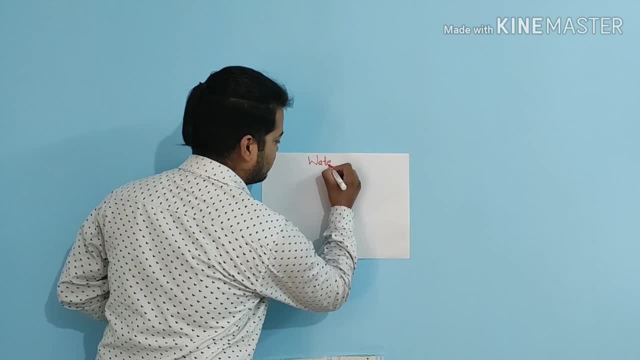 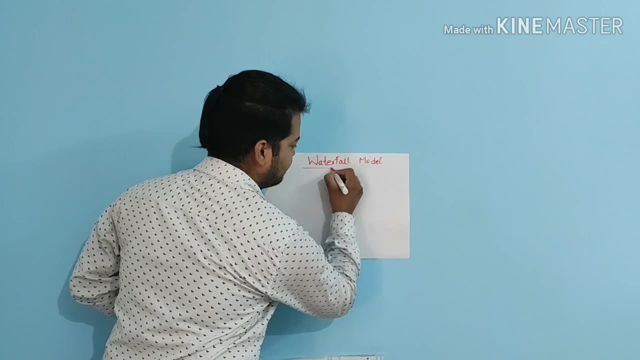 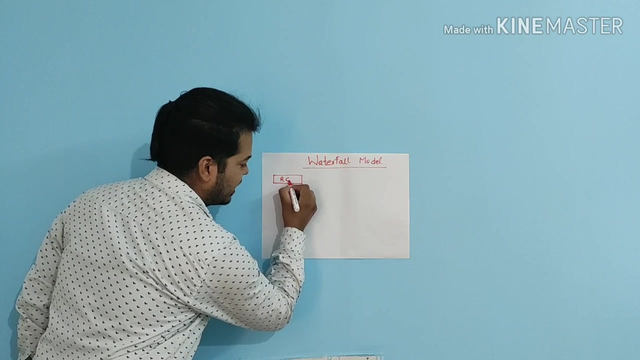 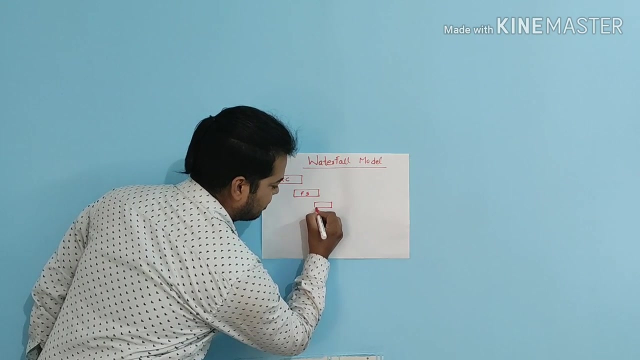 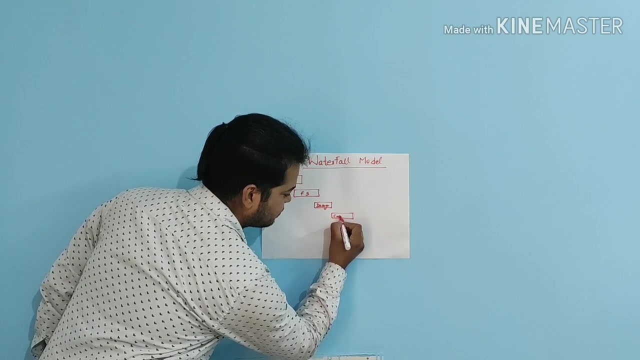 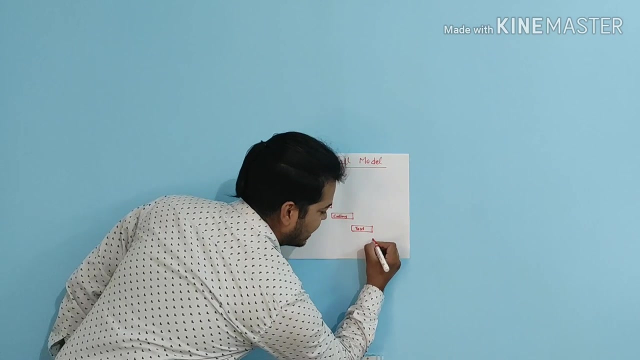 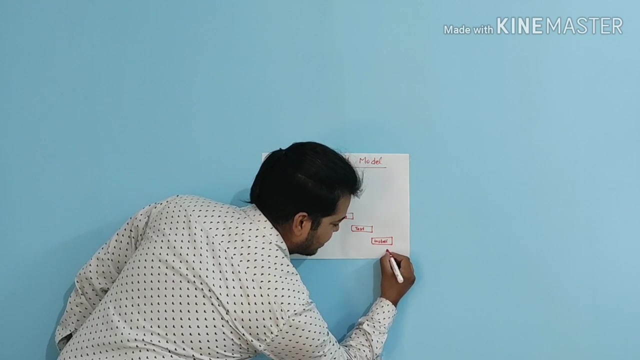 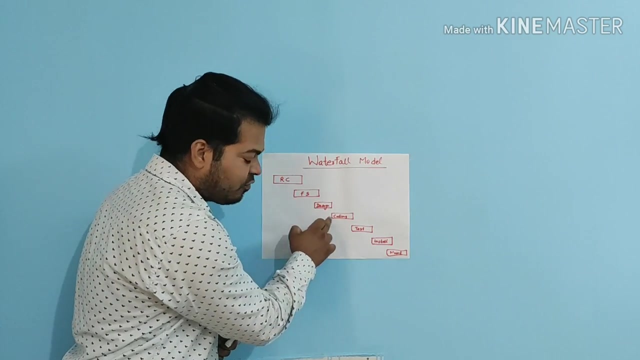 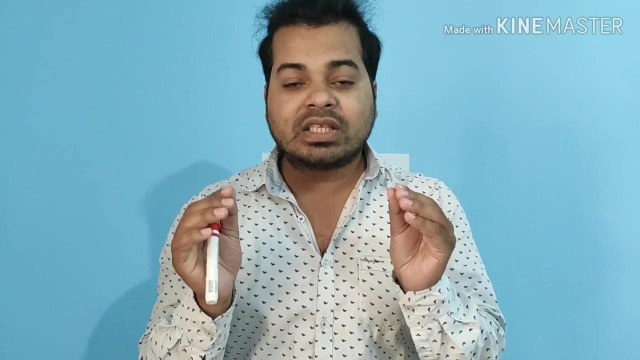 Waterfall model. So in this the first stage is called as requirement collection, Requirement collection, Then comes the feasibility study, Then comes the design, Then comes the coding, Then comes the testing, Then comes the installation, Then comes the maintenance phase. So these are the seven stages of waterfall model. Now I'm going to tell you why. what is waterfall model? 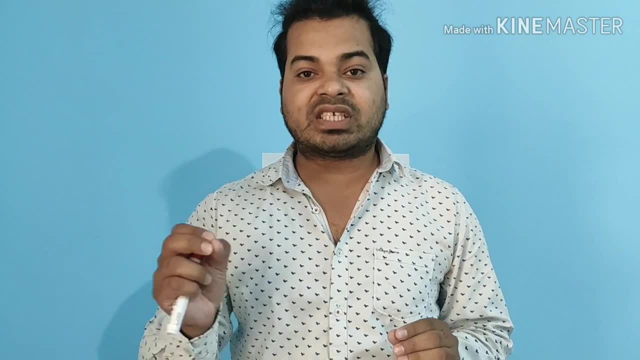 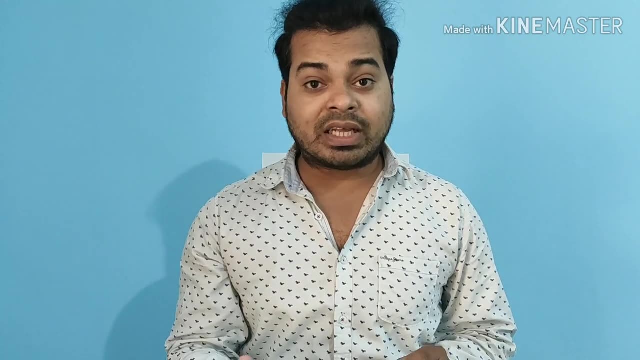 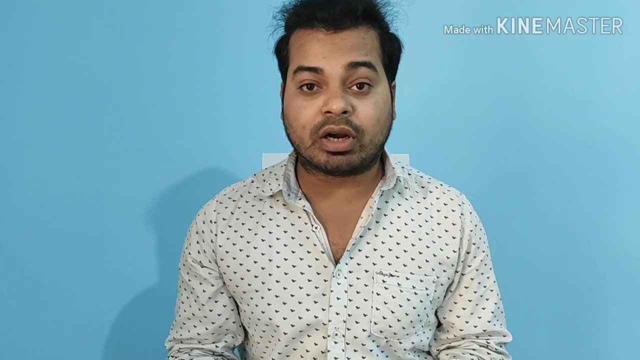 It is a step-by-step procedure or standard procedure to develop a new software. for that purpose we choose waterfall model. It is also called as basic model. It is also called traditional model. It is also called as sequential model. Now how waterfall model is. 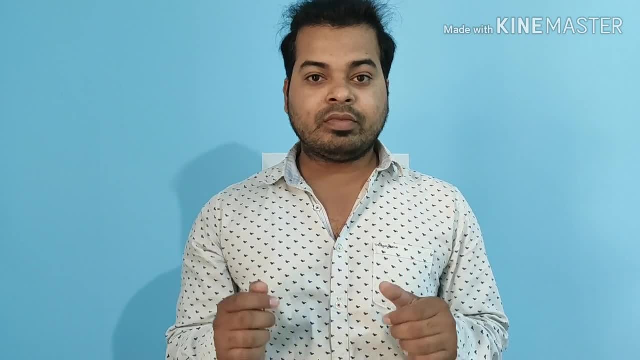 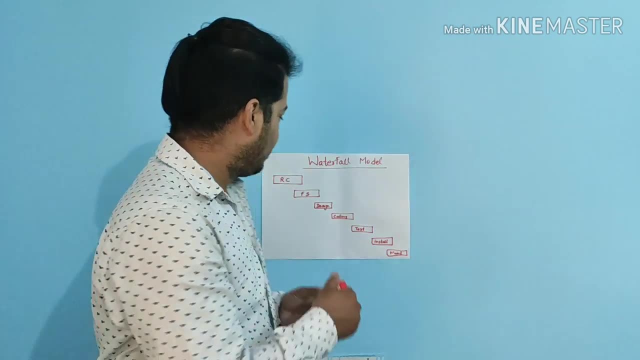 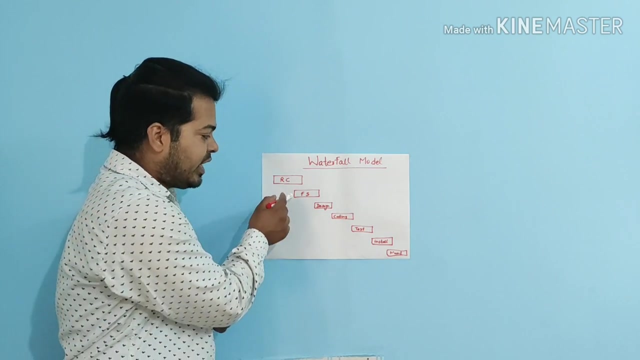 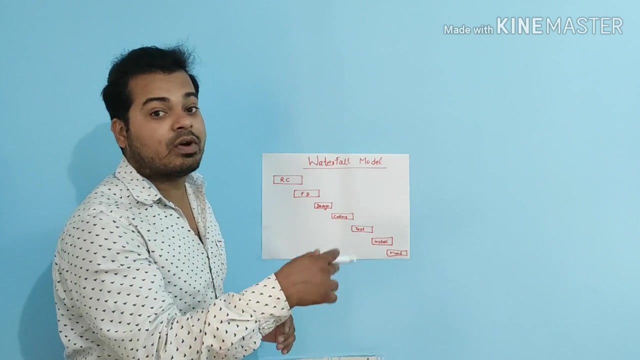 different from other models. In waterfall model will requireonce after the requirement collection is done and feasibility is done, requirement will be freeze. You cannot go back and change the requirement. This is how waterfall model is different from other models. I will tell. 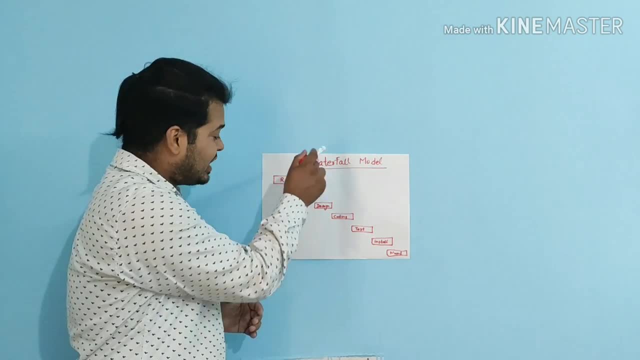 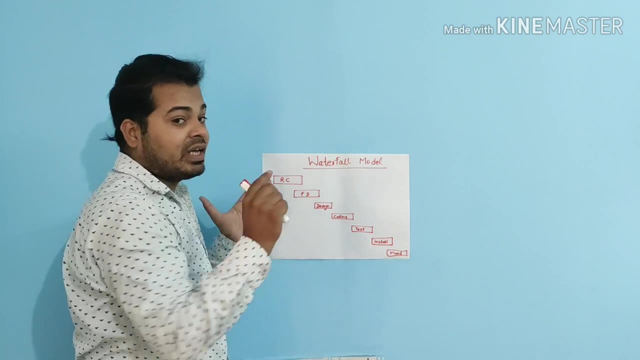 you one more time. Once after requirement, election is done and the feasibility study is done, then requirement will be freeze. You cannot go back and change the requirement. Guys, if you are not understanding what do you mean by all these things, I will request. 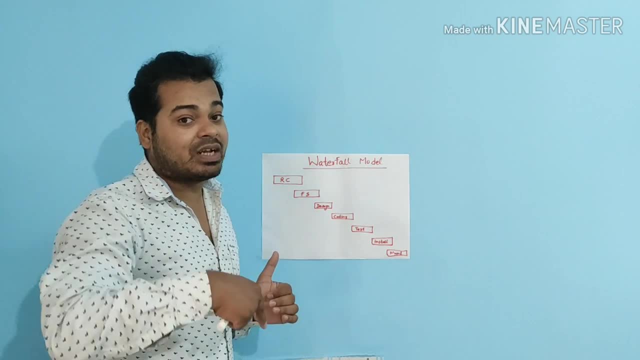 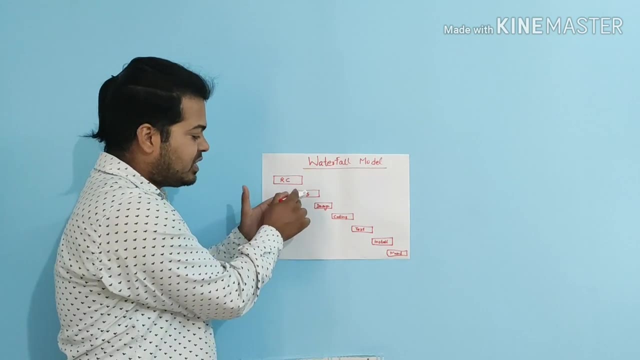 you once again to go back to my software development life cycle video. watch it, then come to this video. So how waterfall model is different from other videos is: once after the feasibility study is done, you cannot go back and change the requirement. Requirement change is not. 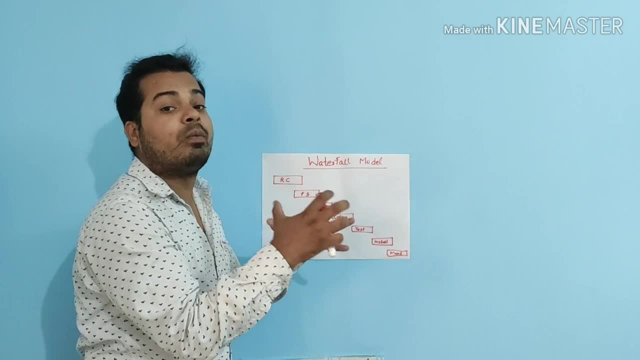 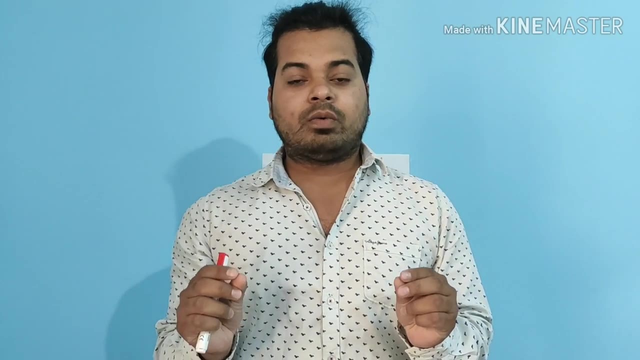 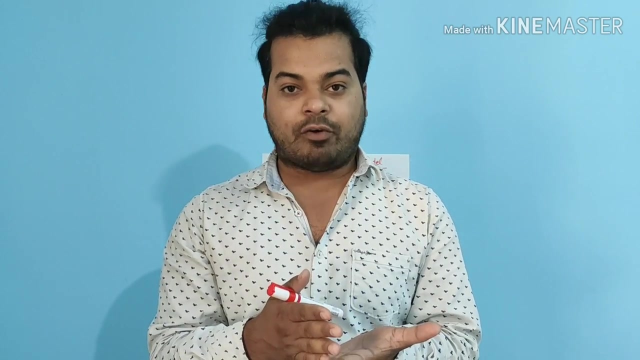 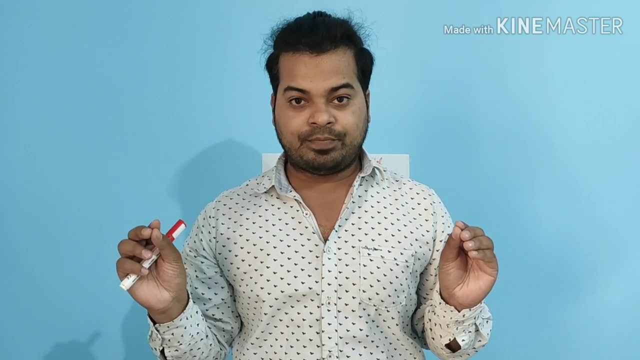 allowed. Once, after the feasibility study is done, it will be freeze. You cannot go back and change it. This is how waterfall model is different from other models. Now what are the disadvantages of choosing a waterfall model? If you choose waterfall model, first disadvantage is requirement. changes are not allowed If and all there is a defect. 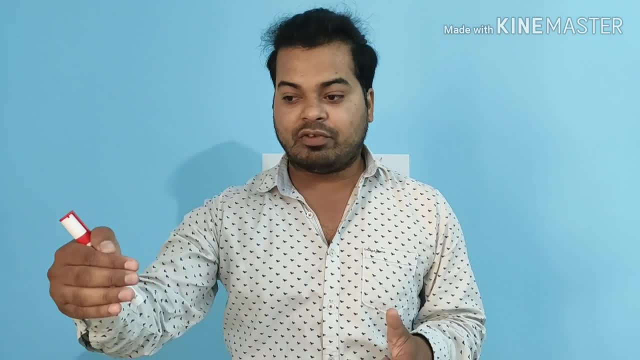 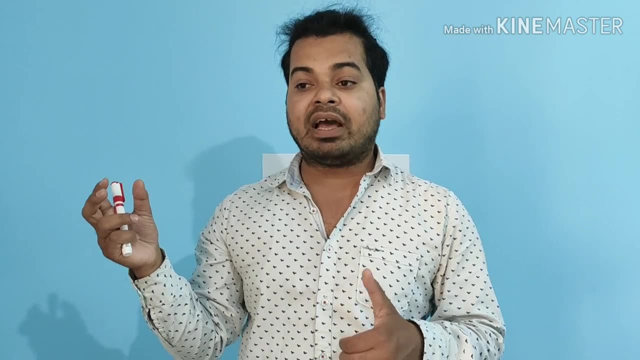 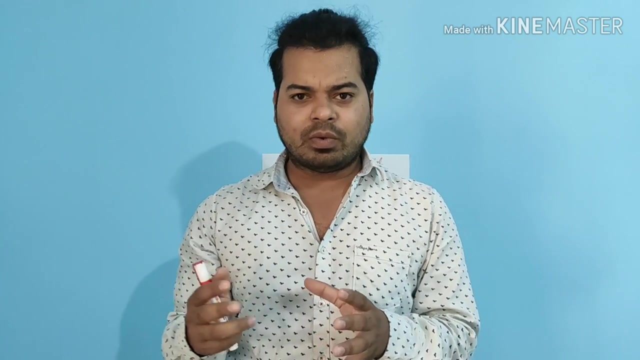 or bug in the requirement, it will flow till design, it will flow till coding and it will flow till software is ready. So we have to put our more effort, starting from requirement collection, then feasibility study, then design, then coding. So if and all there is a defect in the requirement itself, 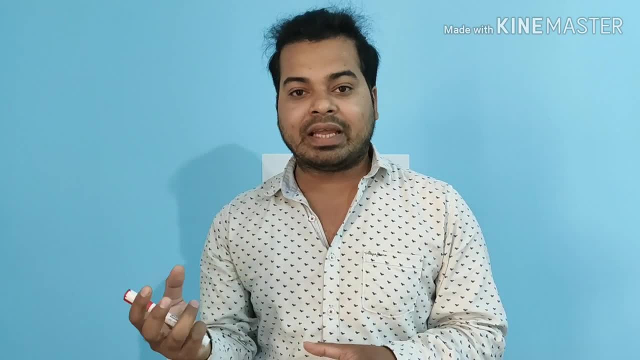 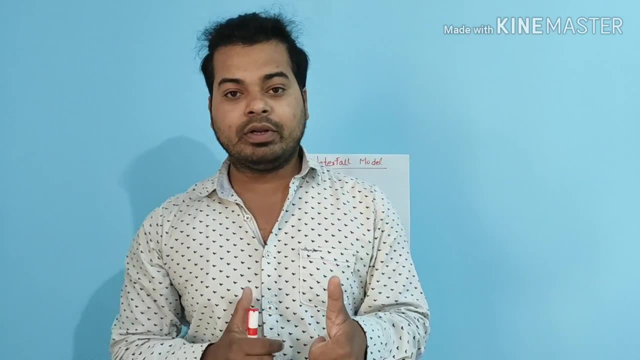 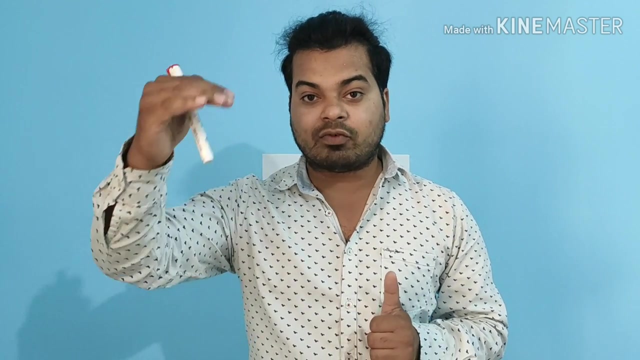 it will flow till end of the software. So total time taken in reworking it it will be more, So time consumption is more. if we take waterfall model, Good, Here total investment is more. How, As I said in the last part, if and all there is a bug in the requirement. 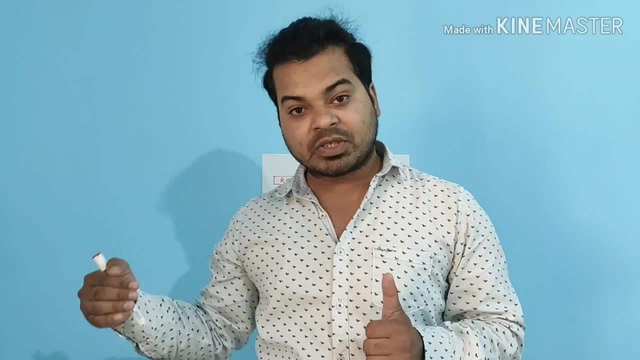 it will flow till design. If and all there is a bug in the requirement, it will flow till design. it will flow till shotgun In the end of the software. So in total time consumption is more. If total time consumption is more, total investment is more. This is. 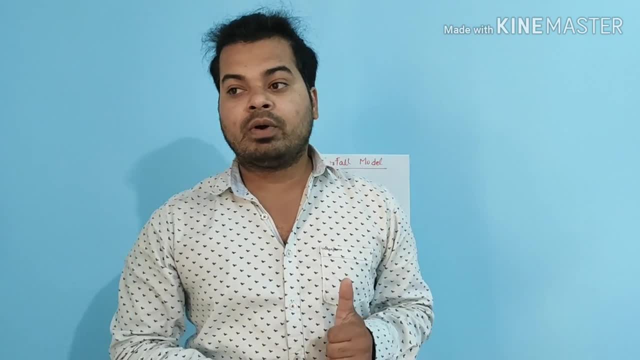 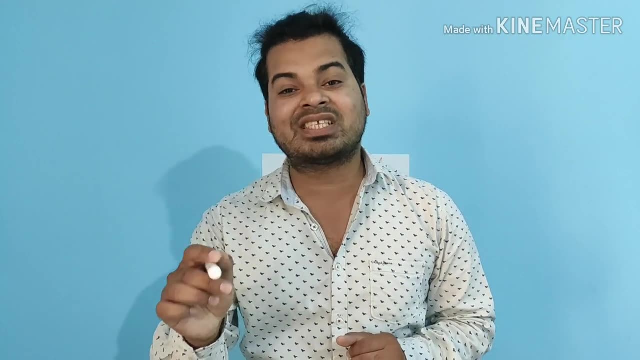 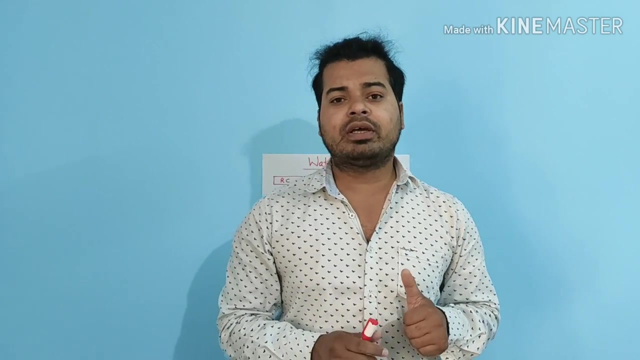 the third point Now. in the biggest disadvantage of waterfall model is here requirement collection in design. the fees aren't tested. Testing will start only after coding. Next point: here also, testers are hired at the later stage of the cycle, So at the later stage of the 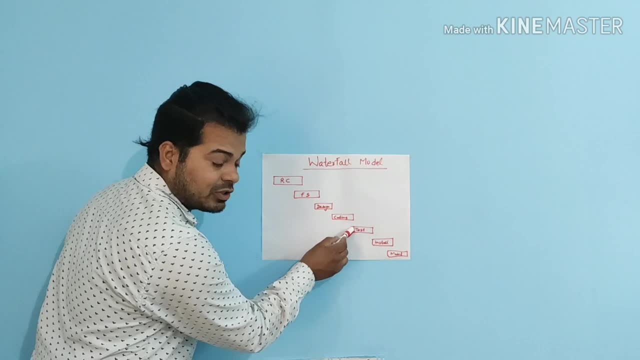 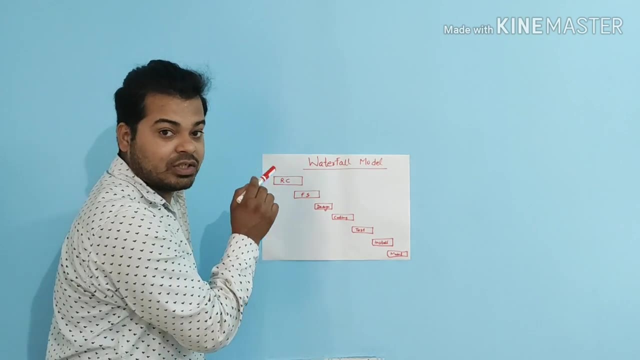 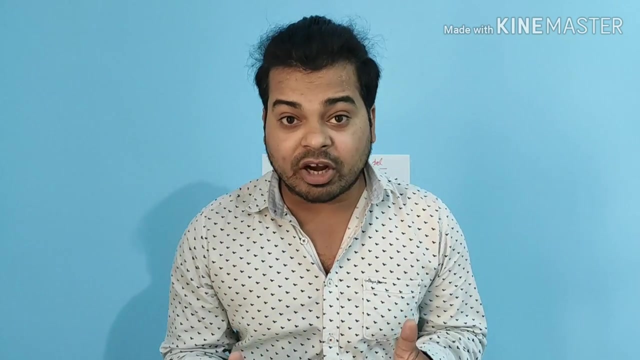 cycle, that is, tourists had to provide testing and then the catch Smooth Teeth software. The testers are hired at the latest in cycle, once after the coding is done, and these are not, these are not tested. so these are the main disadvantage of choosing as a waterfall model and wait for a very long period of time just to see the 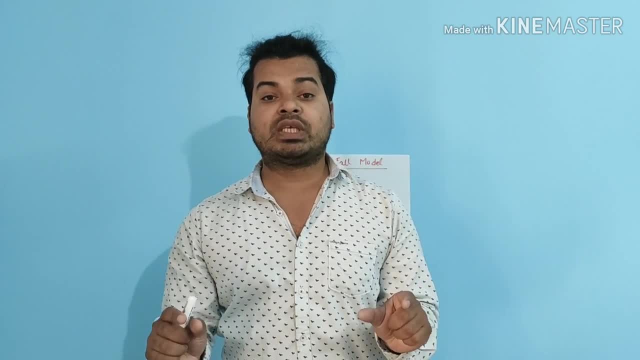 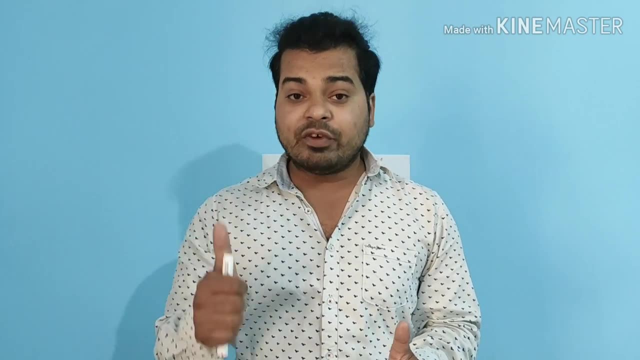 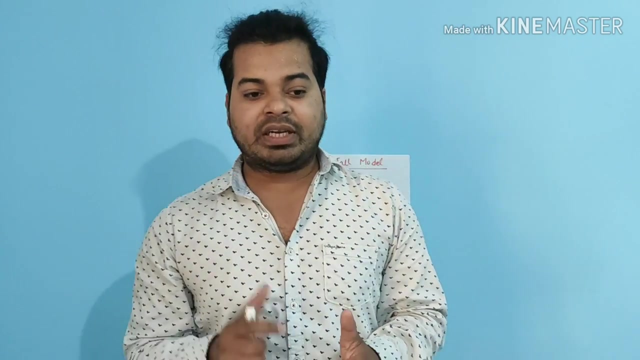 software. so these are the main big disadvantage of choosing our waterfall model. now I'm going to tell you what are the advantages of choosing as a waterfall model. if you are selecting a waterfall model, your quality of the product will be good. first. now the second, since requirement changes are not allowed, chances of finding a bug will be less, and it is an advantage for the developer since he need not record again and again, since the requirement to freeze whatever is developed is ready now. if tester is finding a defect, he needs to fix it. that's all, since the requirement changes. 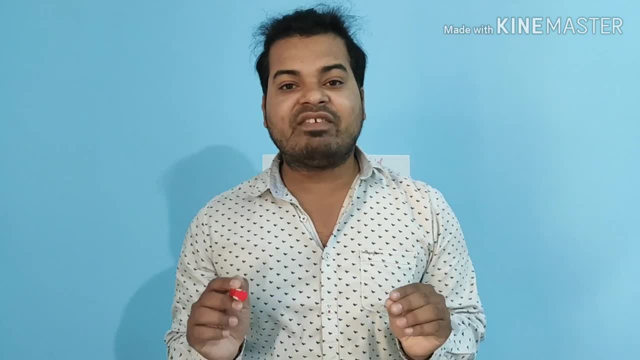 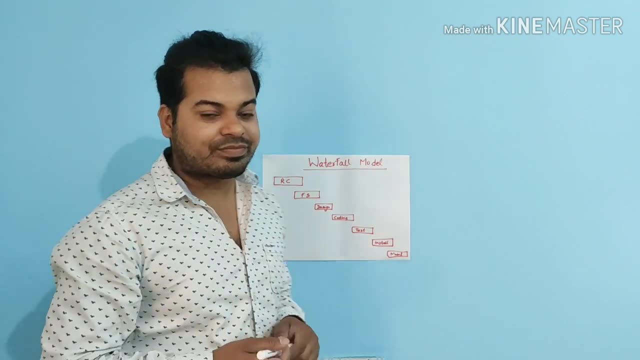 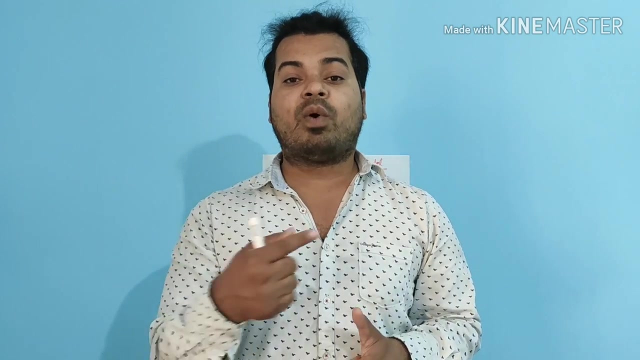 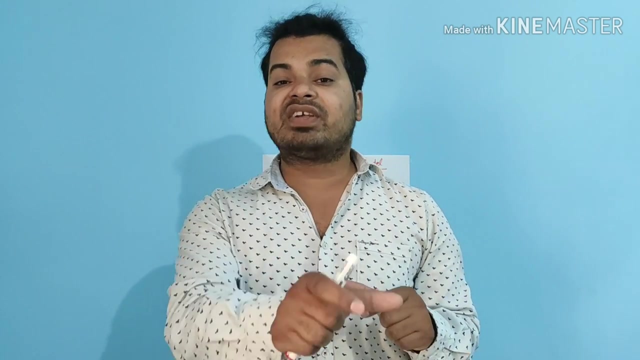 are not allowed. it is the advantage of that initial investment will be less, since the testers are hired at the latest in the cycle. now the question arises for which of projects we should go for waterfall model. so the answer is for small products or where the requirements are. 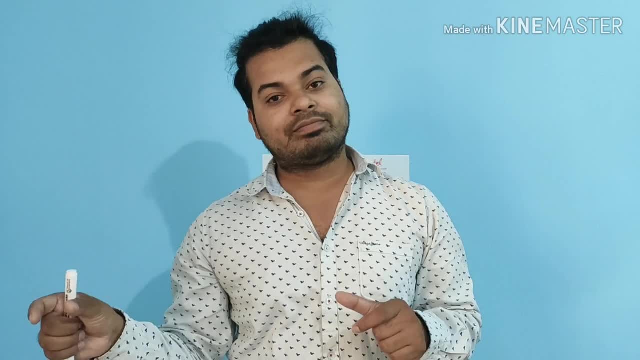 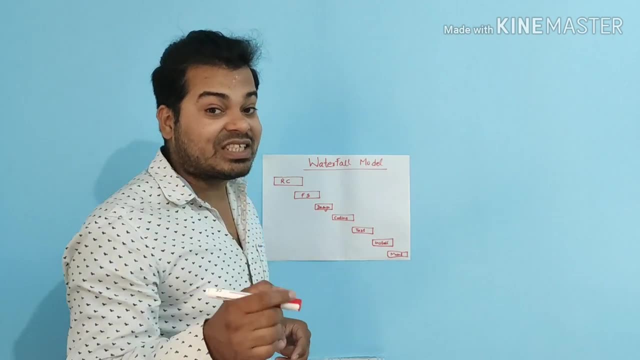 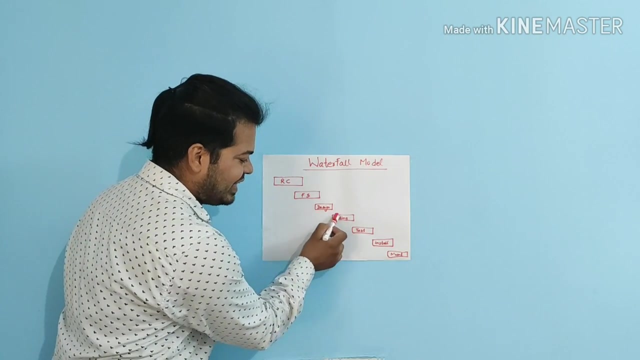 freeze. then we can go for September workflow or further. the requirements will be changed for waterfall model: clear. you must have seen i have drawn waterfall model as like this. now the question arises why? why like this, why not like this? the reason i have drawn waterfall model like this once: after economy collection system we do feasibility study once. 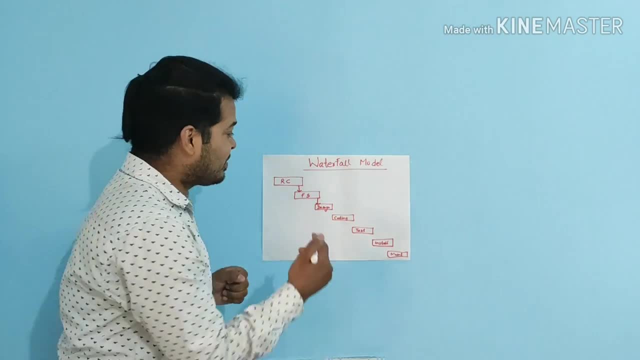 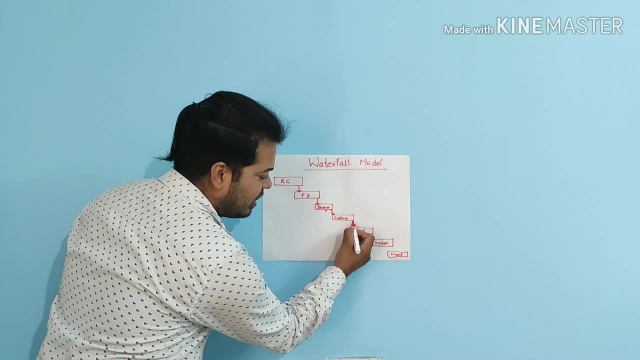 after feasibility is done we do design. and i have said already, in waterfall model, backtracking is not possible after feasibility study. so after design we do coding. after coding, we do testing, after testing we do install and then we do maintenance. now the question is why i have 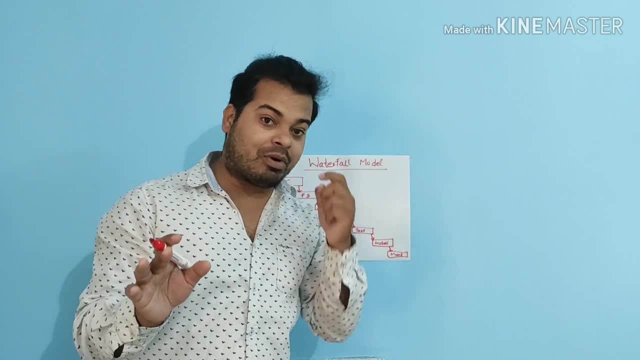 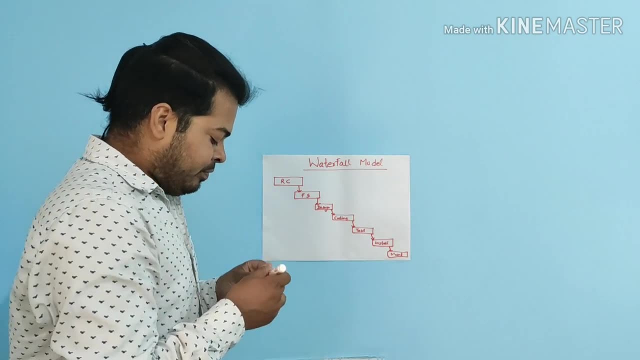 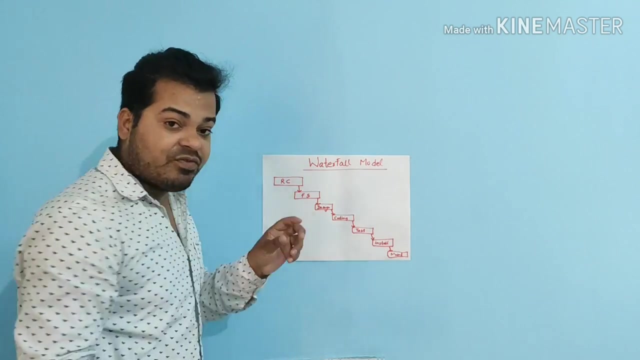 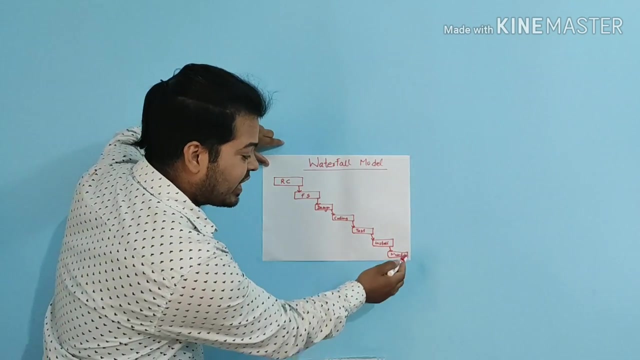 drawn like this. see, guys, wherever you see waterfall model picture, you will get it this way. now question is: the reason is. understanding is very easy, guys. let's suppose these are the steps. if you try to pour a water on top of it, it will go till end and water cannot come from end to the top in a similar way. 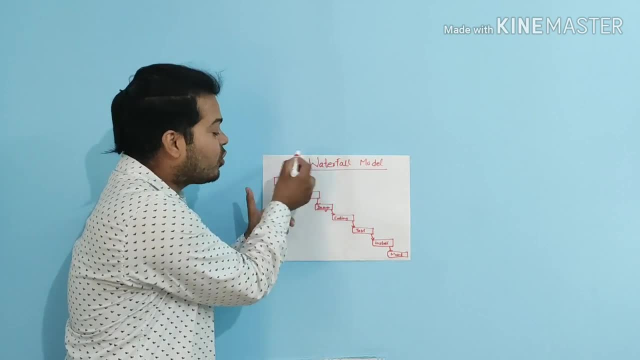 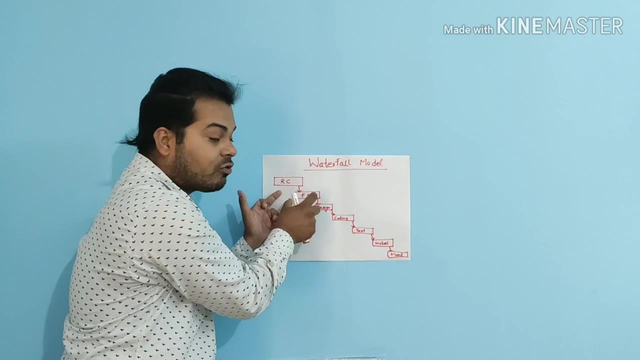 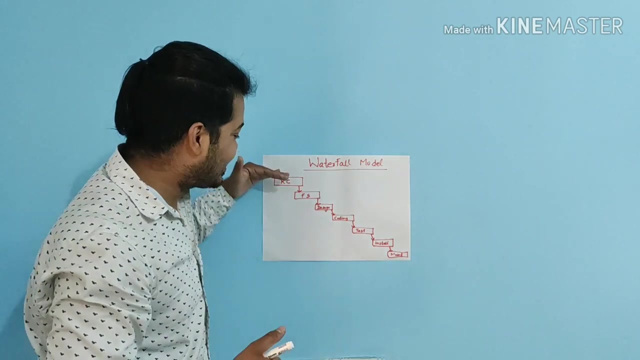 once after the feasibility study is done, you cannot go back. you have to go only in this direction. once after requirement collection is done, feasibility study is done, requirements are freezed. you cannot go back and change the requirement. you have to proceed like this. that's why it is called as waterfall.